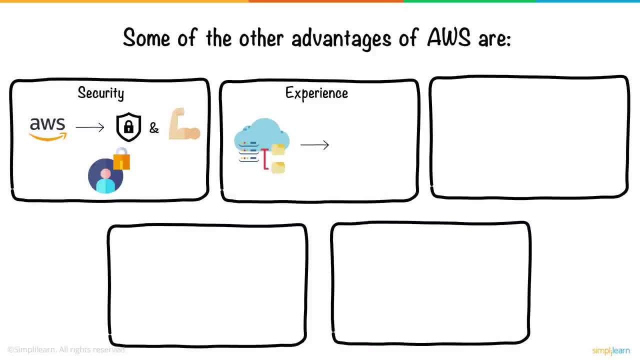 You can benefit from the infrastructure management practices born from Amazon's years of experience. Flexible: It allows users to select the OS language database and other services. Easy to use: Users can host applications quickly and securely. Scalable: Depending on user requirements: applications can be scaled up or down. 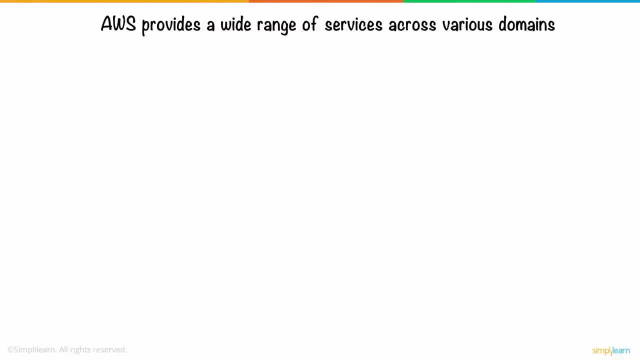 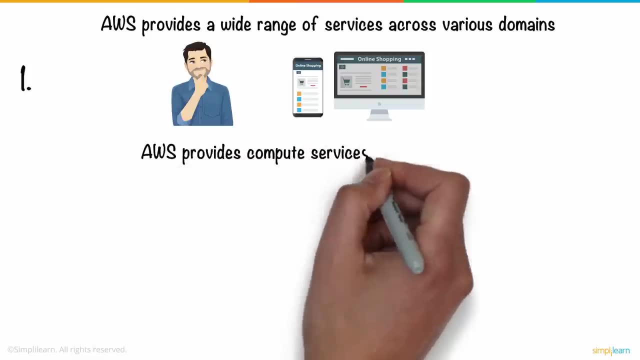 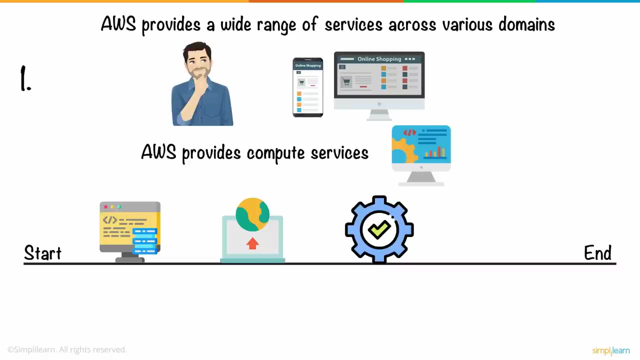 AWS provides a wide range of services across various domains. What if Rob wanted to create an application for his online portal? AWS provides compute services that can support the app development process from start to finish, From developing, deploying, running to scaling the application up or down based on the requirements. 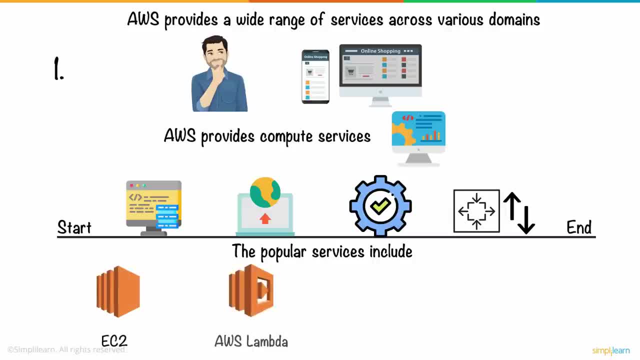 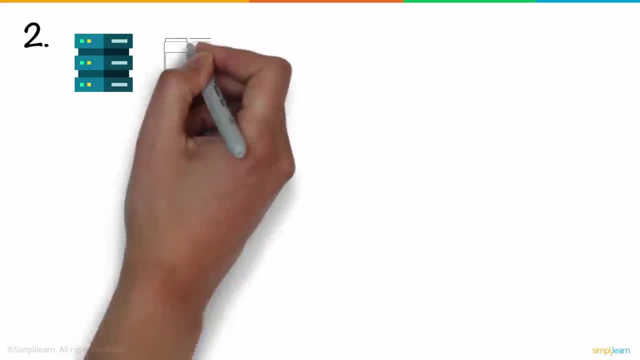 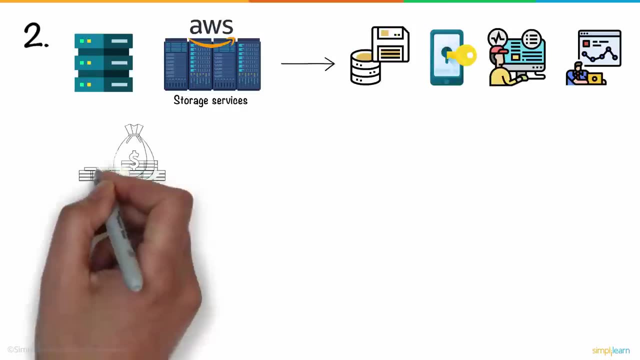 The popular services include EC2, AWS, Lambda, Amazon LightSell and Elastic Beanstalk For storing website data. Rob could use AWS storage services that would enable him to store, access, govern and analyze data. to ensure that costs are reduced, Agility is. 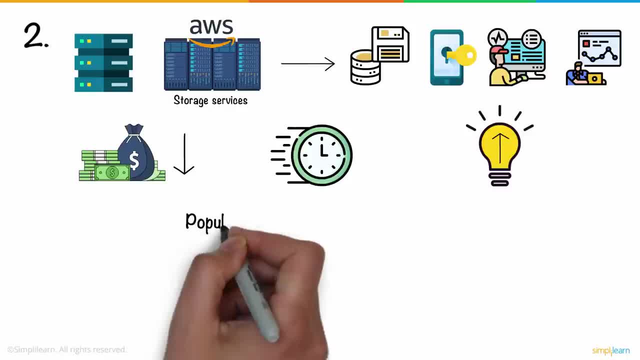 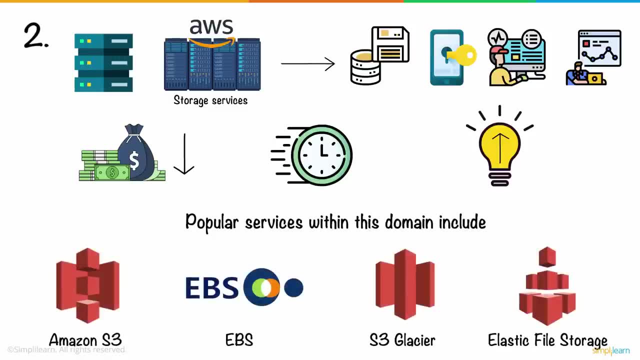 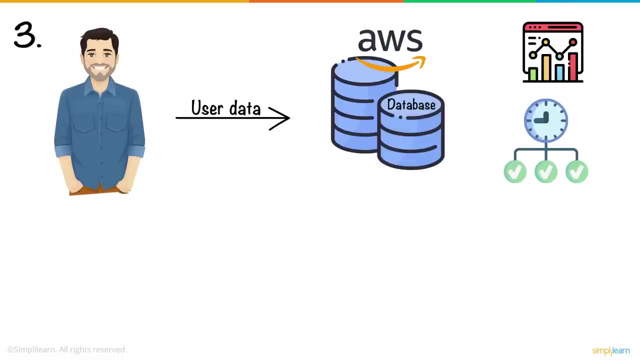 improved and innovation accelerated. Popular services within this domain include Amazon S3, EBS S3, Glacier and Elastic File Storage. Rob can also store the user data in a database with AWS services, which he can then optimize and manage. Popular services in this domain include Amazon RDS. 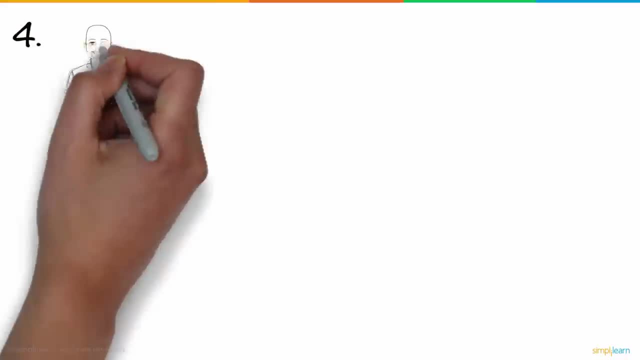 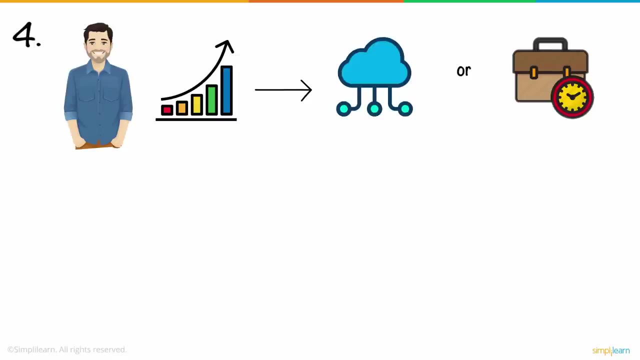 DynamoDB and Redshift. If Rob's businesses took off and he wanted to separate his cloud infrastructure from the rest of the world, he could use AWS storage services. If he wanted to scale up his work requests and much more, he would be able to do so with the networking. 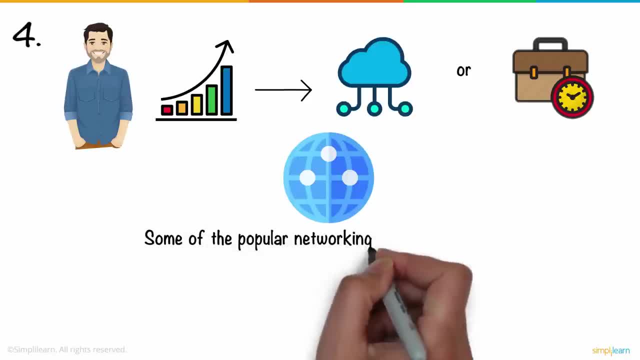 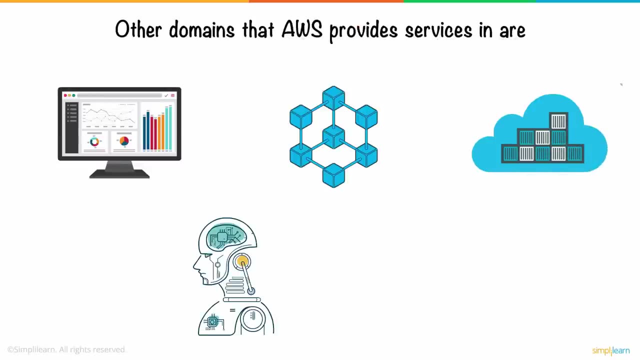 services provided by AWS. Some of the popular networking services include Amazon VPC, Amazon Route 53, and Elastic Load Balancing. Other domains that AWS provides services in are analytics, blockchain, containers, machine learning, Internet of Things and so on. 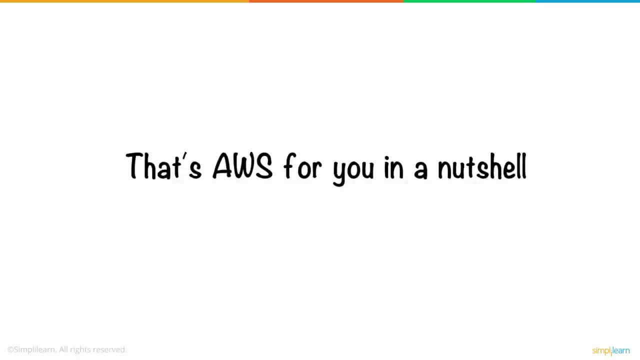 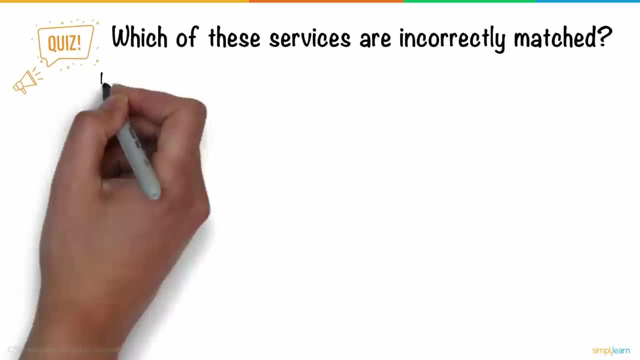 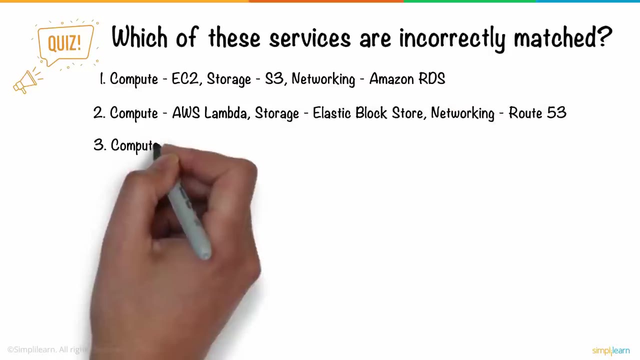 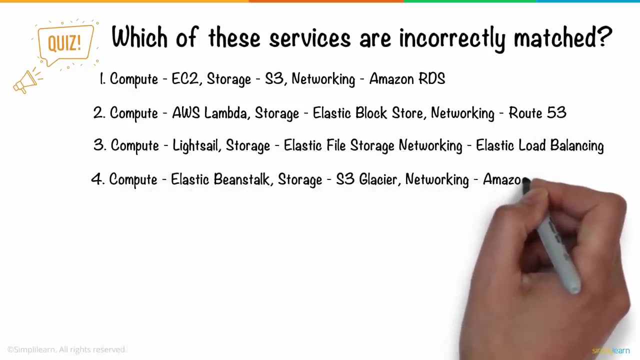 And there you go. That's AWS for you in a nutshell. Now, before we're done, let's have a look at a quiz. Which of these services are incorrectly matched? We'll be pinning the question in the comment section. Comment below with your answer.